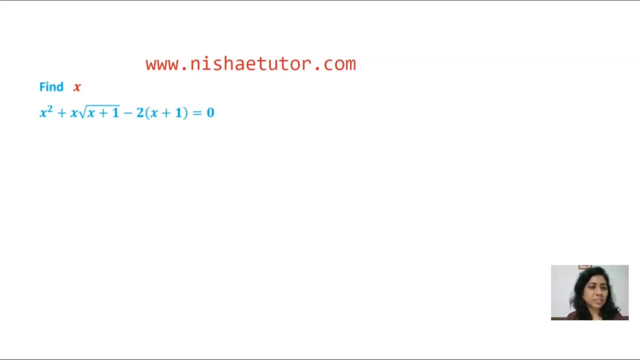 Namaste. in this video we are going to simplify this problem for x Here. given x square plus x, square root x plus 1 minus 2, x plus 1 is equal to 0. This question looks difficult but very easy if you follow these steps. Here this part, square root x plus 1, we can write a- is equal to. 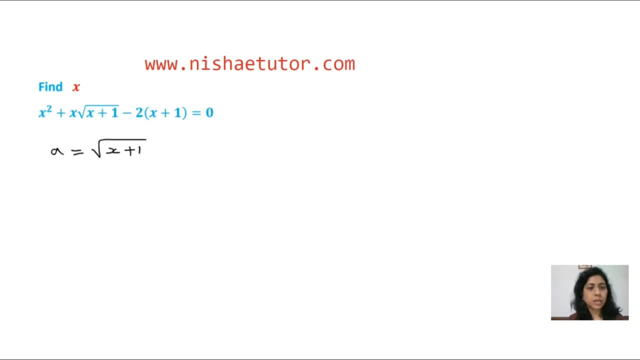 square root x plus 1, and this is more than 0, it means positive, So A square, both side taking squares. So this is x plus 1 and when we find out x value, So A square minus 1 is equal to x or x is equal to A square minus 1.. This equation we can convert into: 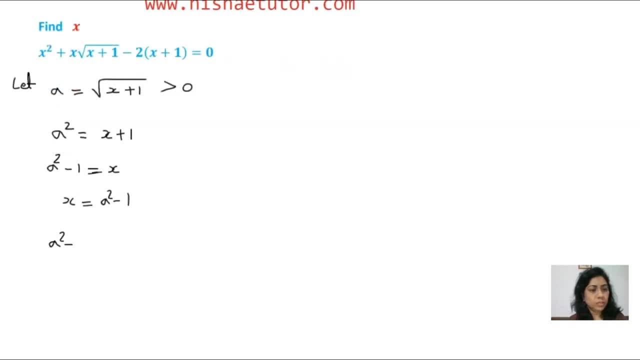 a form, so a square minus 1. we can substitute x value and here x value when we substitute. so a square minus 1 and this square root x plus 1, is a minus 2. here x plus 1 value is a square is equal to 0. we can simplify this. here we can apply a minus b, whole square form. 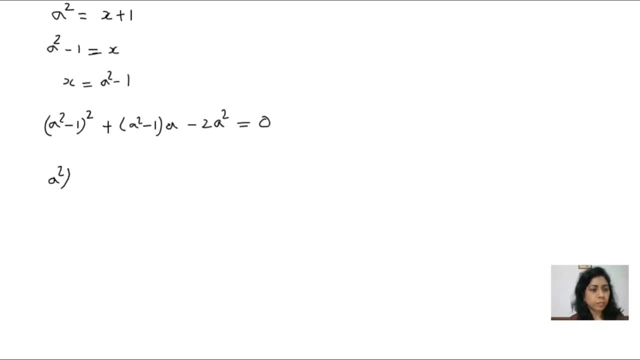 algebraic identity. so a square, this square minus 2, a square multiply 1, so just this value plus 1 square, it means 1. and when we simplify this parenthesis, so here: a square multiply a, a cube minus 1, multiply a minus a minus 2, a square is equal to 0, a to the power 4. 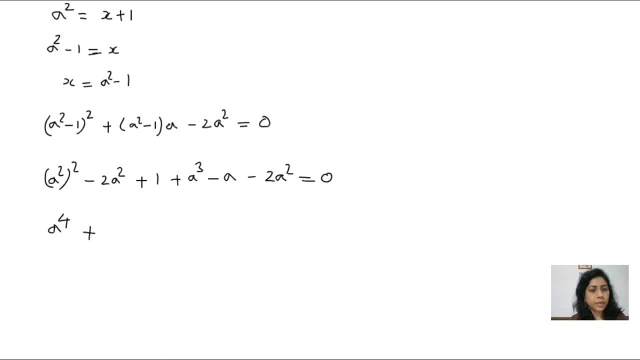 and we can rearrange and combine like terms: a to the power 3. then minus 2 a square, minus 2 a square will be minus 4. a square minus a plus 1 is equal to 0. this term and this term we can combine. this is a to the power 4 and we want to convert into: 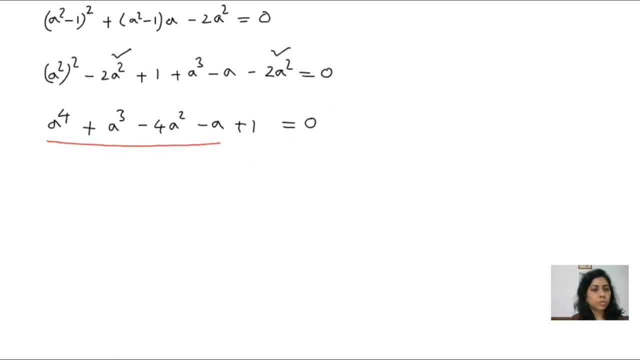 quadratic form. so so, both side, divided by a square a to the power, 4 divided by a square, a square plus a cube. divided by a square a minus 4, a square divided by a square 4 minus a, by a square minus 1 upon a, and here, 1 divided by a square is equal to 0.. 0 divided by any number. 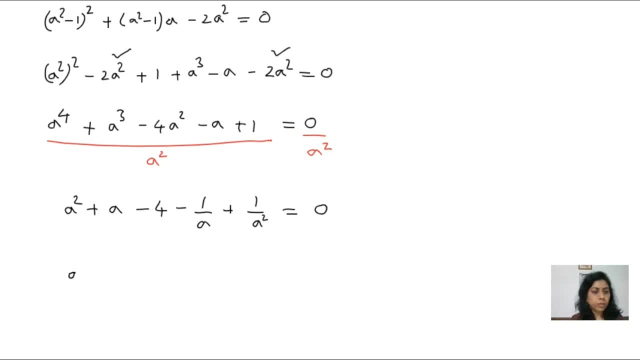 always answer 0. This one we can rearrange and make perfect square number. So for this a square and this last term we can write here, and then this one: a minus 1 upon a, and minus 4 is equal to 0. So here you can see this one a minus 1 upon a. If we make this one a minus 1 upon a, 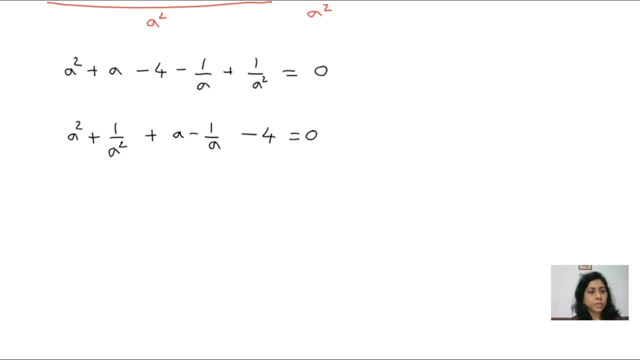 square, whole square. So for that here we have to subtract 2.. So 1 upon a square minus 2, and here a minus 1 upon a. Here we wrote minus 2.. So we can write here minus 2, because minus 2 and minus 2 is minus 4.. And this one we can write a minus 1 upon a. 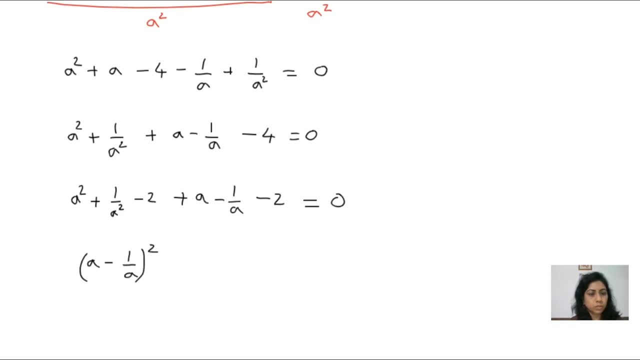 whole square. This is perfect square, okay, And here a minus 1 upon a minus 2 is equal to 0.. Here again we let y. another variable is equal to a minus 1 upon a, So this will be y square minus y. actually, plus y minus 2 is equal to 0.. And this is quadratic. 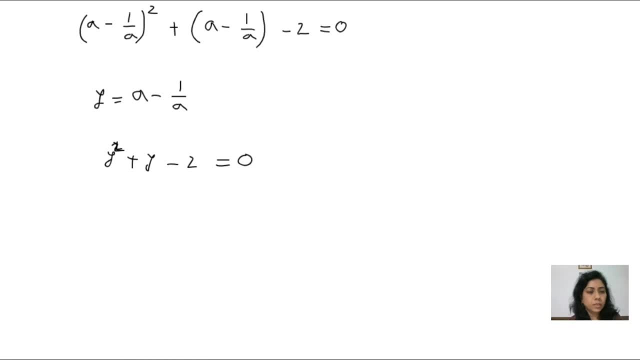 equation And we can easily here factorize this quadratic equation Here: product is minus 2 and sum is 1.. So we choose 2 numbers: 2 times minus 1 is minus 2, and 2 minus 1 is 1.. 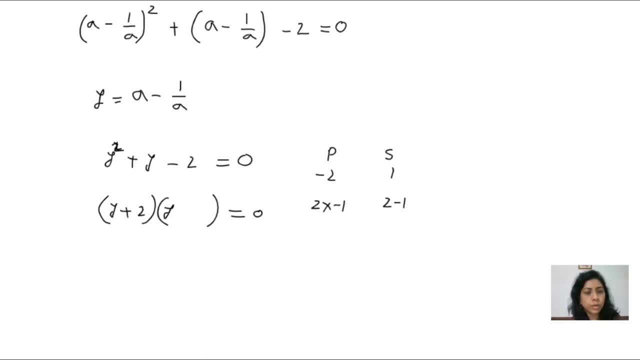 So we got 2 numbers, plus 2 and minus 1.. So y plus 2 is equal to 0.. 0 or y minus 1 is equal to 0.. y is equal to minus 2, we got this y value and here 1. And 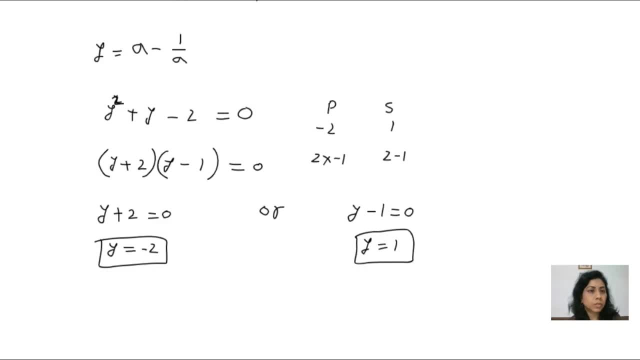 what is y value Here? this one a minus 1 upon a. So we can substitute: here a minus 1 upon a is equal to minus 2, here a minus 1 upon a is equal to 1.. We can simplify this. 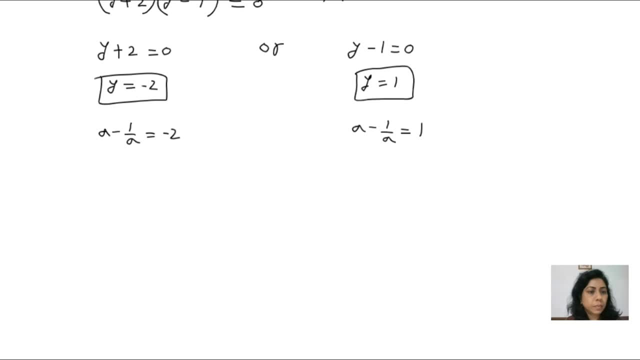 one first. So whole equation multiply by a, So it will be a square. minus 1 is equal to minus 2a, and all these terms shift left side So it will positive: 2a minus 1 is equal to 0. And this quadratic equation we cannot solve. 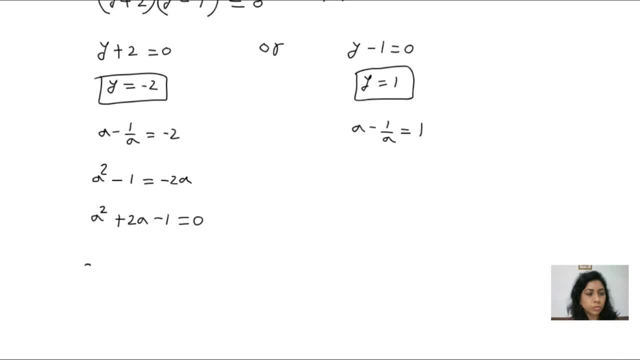 by factorizing method. So we can use here quadratic formula, Here a value. if we compare this: x square, ax square plus bx plus c, So here a value 1, b value 2 and c value minus 1.. So minus b, which is 2 plus minus square root, b square it means 4 minus 2.. So we 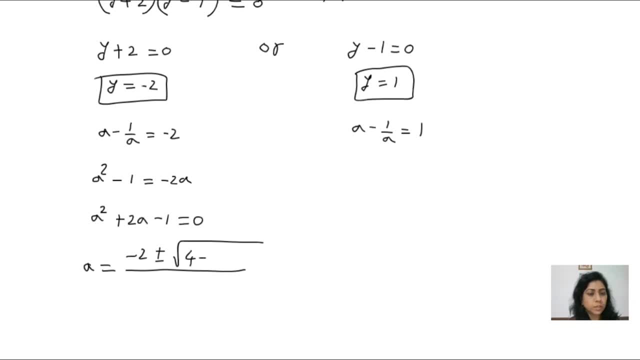 have 4, this is 2 square is 4 minus 4, a value 1, c value minus 1 divided by 2, a value 1.. So minus 2 plus minus here, this is minus 4 times minus 1, is 4, 4 plus 4, 8 and divided. 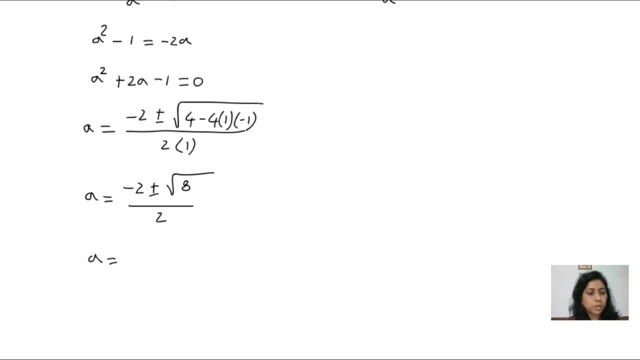 by 2 times 1, 2. So we can take common 2 or here divide by 2.. So minus 2 divided by 2 is minus 1 plus minus and square root 8 is 2, square root 2.. So 2, 2 cancel just square root 2. So 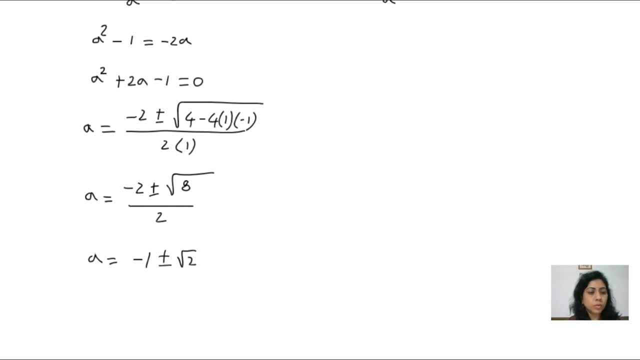 here we got two values: minus 1 plus square root 2 or minus 1 minus square root 2.. But in earlier here we let: this is positive, So negative we can just negligible this, So we can take only positive number which. 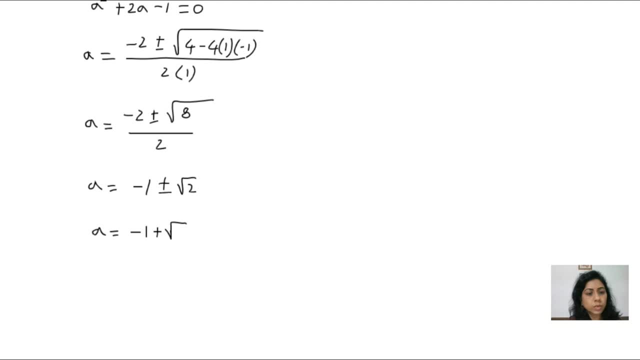 is minus 1 square plus square root 2, or we can say square root 2 minus 1, this is a value okay. Now here second equation. this we can solve Here. multiply by A, so this is A square minus 1, is equals to A 1 times A. A, A square- 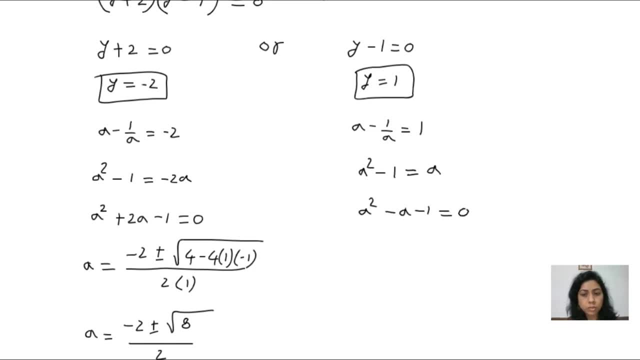 minus A minus 1 is equals to 0.. Here again we apply this quadratic formula: minus b-value, here minus 1, plus minus square root 120.. editorial minus 1, square minus 4, a value 1, c value minus 1 divided by 2, a value 1.. So what is a value? 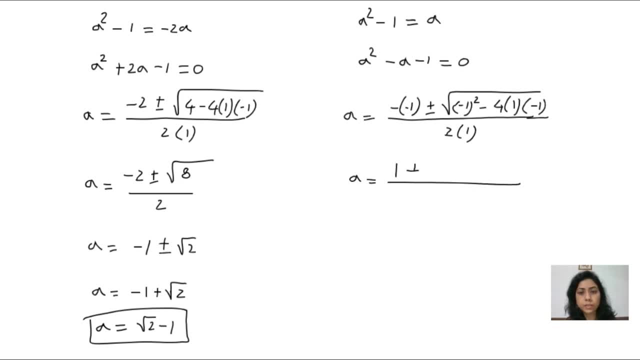 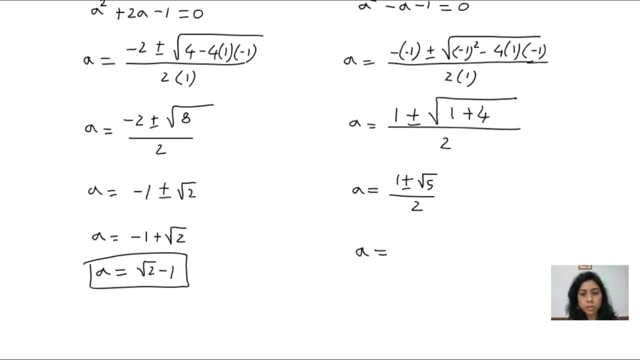 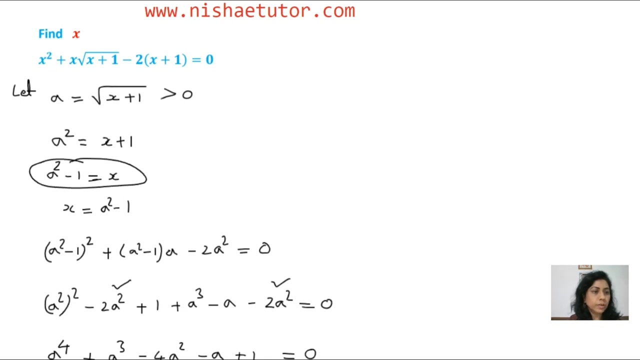 Okay, minus minus plus, plus minus 1 plus 4 divided by 2.. So here a 1 plus minus square root 5 divided by 2. and again here we want positive. So just this one: 1 plus square root 5 divided by 2.. Okay, because a is positive and final we have to find out x. So here: 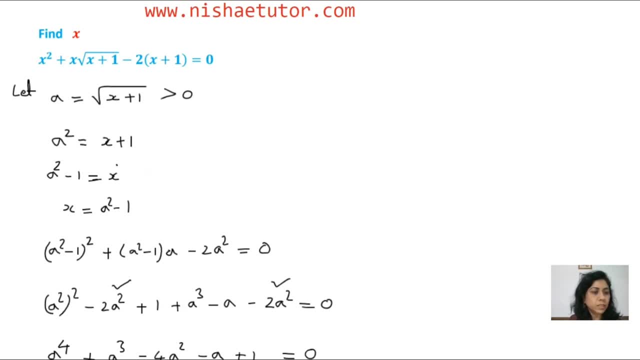 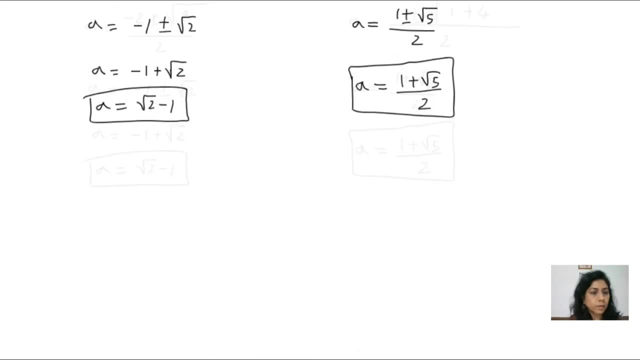 if we find out a square and minus 1.. So we can easily find out x. So for a square root, first square, it a value, a square, both side, taking square root 2 minus 1 square, Okay. here also a square is equal to 1 plus square root 5 divided by 2, whole square: Okay. so 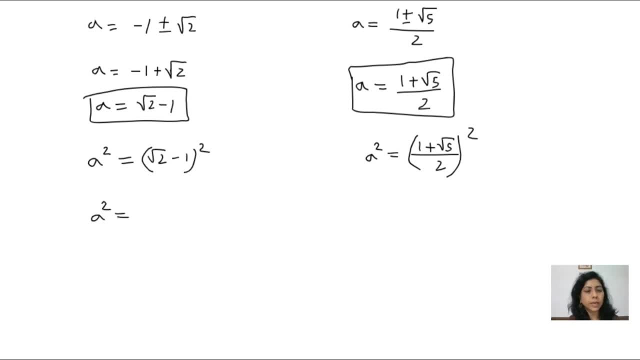 what is a square value? Here we can apply algebraic identity: a minus b, whole square formula. So square root 2 square minus 2, a value square root 2, b value 1 and here 1 square. Okay, so here square root 2 square is 2 minus 2. square root 2 plus 1. 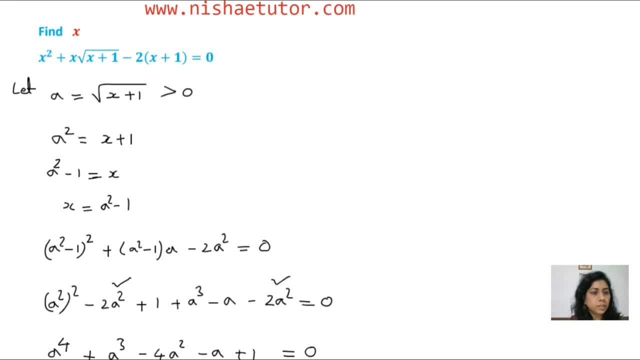 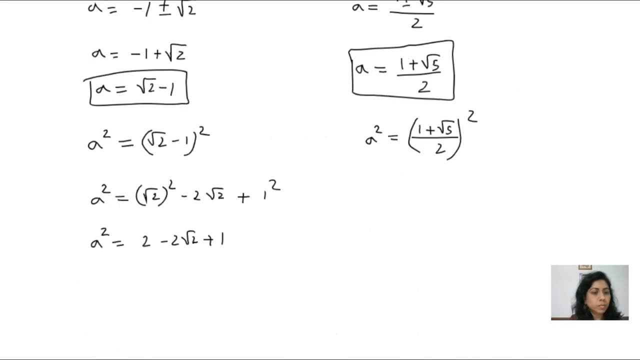 and we want a square minus 1, right, a square minus 1.. So we will get x. So we can here write a square and 1 transfer here. So this is 2 minus 2, square root 2 and this is x value right, This a square minus 1. we can write x and here we can take common 2. 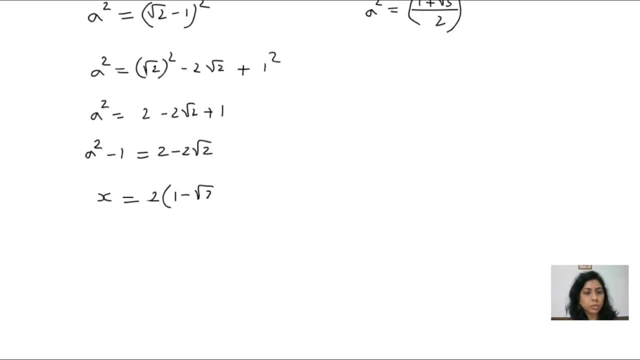 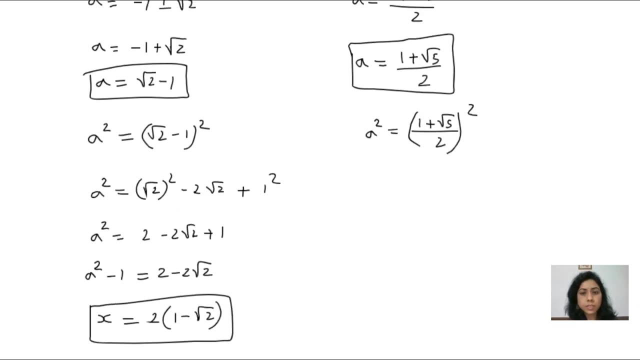 here 1 minus square root 2.. This is our final answer, one final answer, And here we can solve this: a square, here 1 plus square root 5, whole square. So 1 square plus 2 a value, 1 b value, square root 5 plus square root, 5, square, and here 2 square, which is 4.. 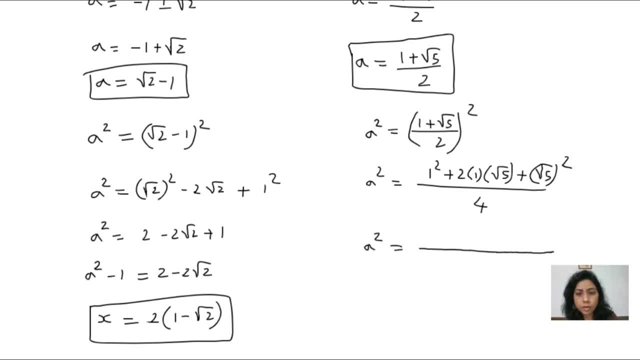 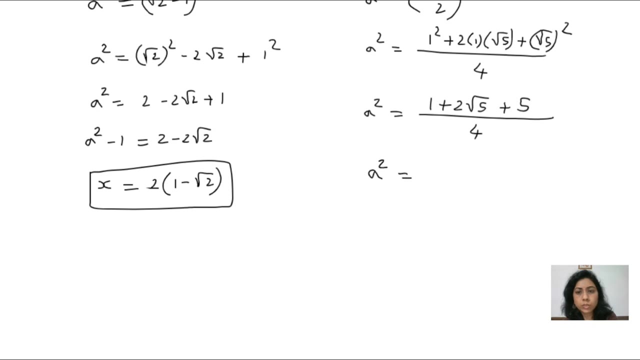 A square value here: 1 plus 2 square root 5 plus square root 5, square is 5 divided by 4.. a square is equal to 6, 1 plus 5, 6, 2 square root 5 divided by 4.. So we can take common 2.. So this is: 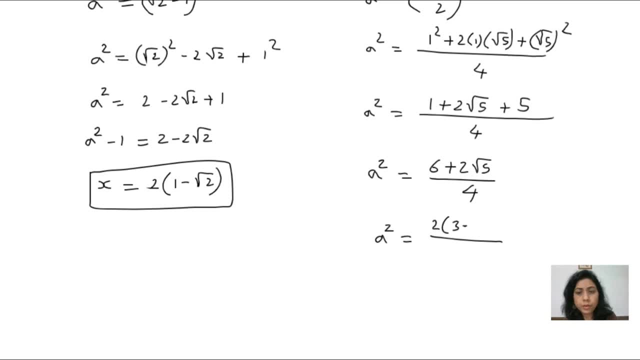 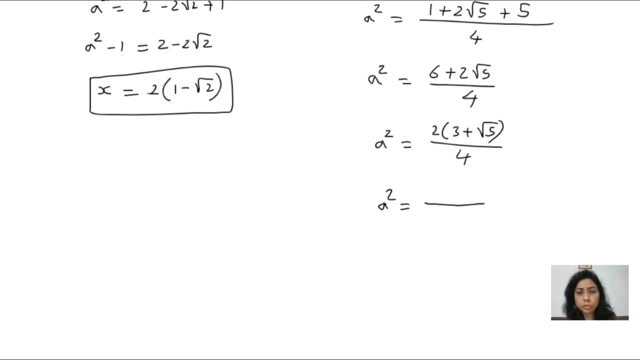 2, 3 and square root 5. here 4, now 2 and 4 cancel. So this is 3 plus square root 5 divided by 2.. Okay, and we want a square minus 1, because this is x value. So 3 plus square root 5 divided by 2.